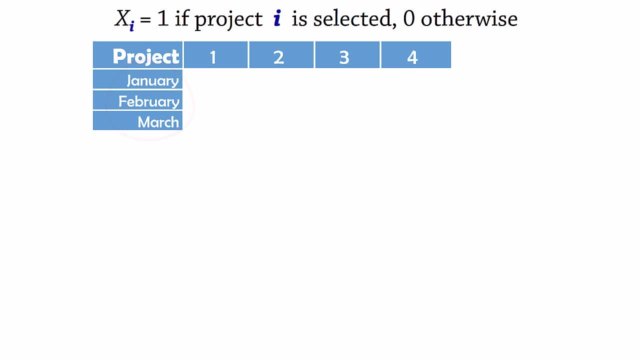 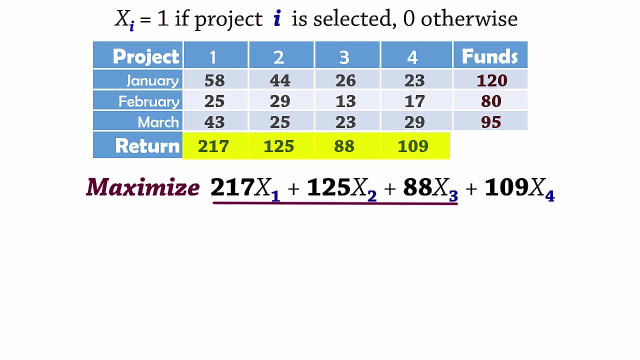 to merge with corresponding outlays or costs in thousands of dollars shown here. Suppose these are the funds available for selected projects each month and these are the net returns in thousands of dollars from each project. In this case, our objective is to maximize return, which is 217x1 plus 125x2 plus 88x3. 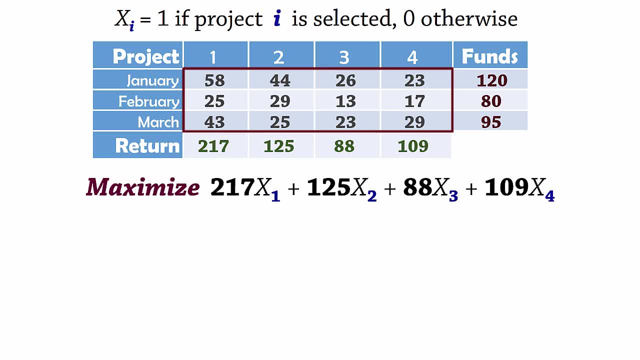 plus 109x4.. Since project outlays are constrained by available funds, we write for January: 58x1 plus 44x2 plus 26x3 plus 23x4, less than or equal to 120.. We do the same for February and for March. 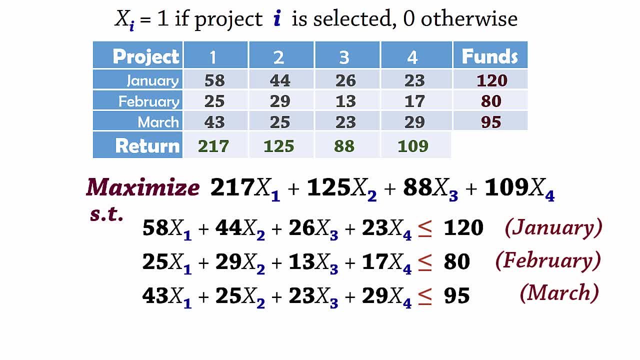 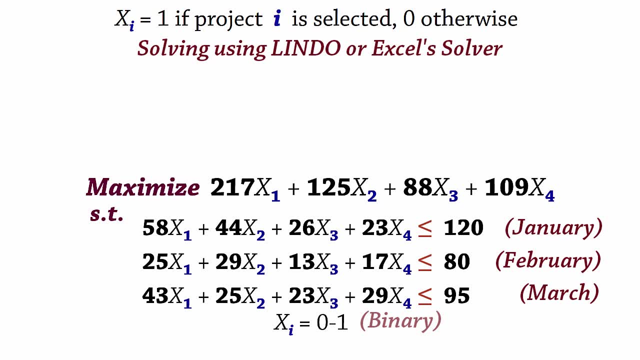 And then complete the model by stating that the decision variables must be binary. Upon solving this model using software like Lindo or Excel Solver, we find that the optimal solution is: x1 equals 1.. x2 equals 0, x3 equals 1, and x4 equals 1, with a corresponding net return of 414. 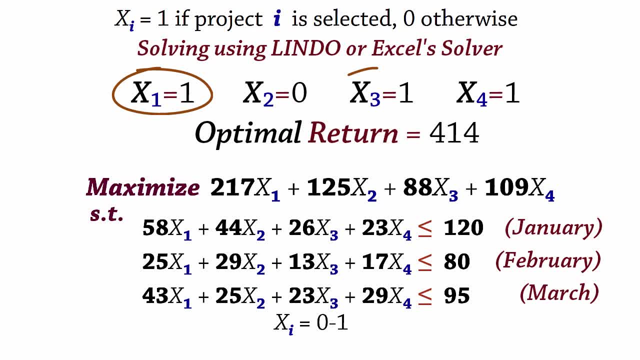 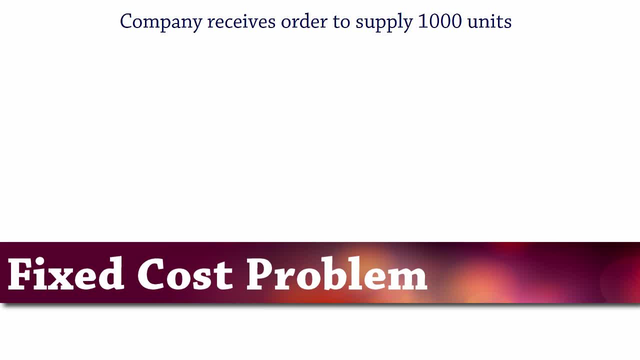 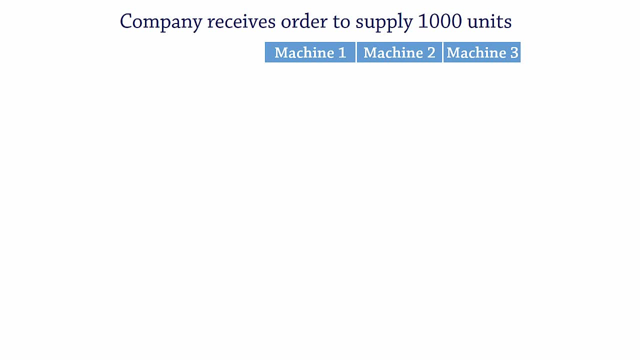 That is, to maximize net return. undertake projects 1,, 3, and 4 only. Let's now model a fixed cost problem. Suppose a small company receives an order to supply 1,000 units of a product. The company has three machines that can be used to produce the product. 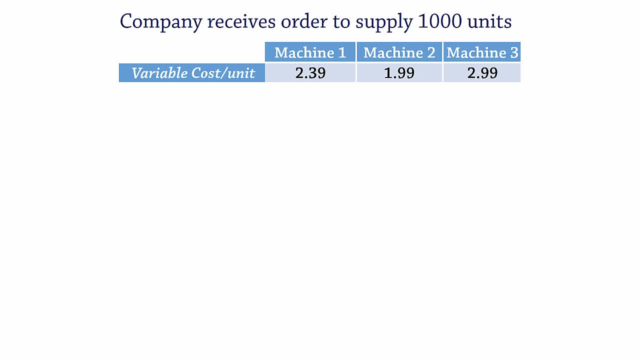 Here are the variable costs per unit produced from each machine, Here are the fixed costs And here are the machine's capacities. Our objective is to minimize total costs. We are going to need two types of decision variables in this case: One set for the number of units produced from each machine and because of the fixed costs. 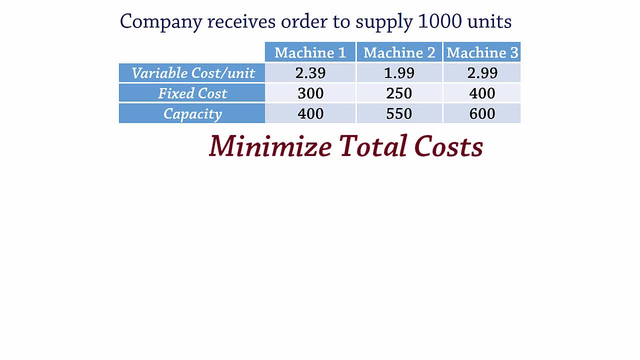 another to indicate whether a machine is being used or not. So for the units produced we write: x1 equals number of units produced on machine i. That is, x1 represents the units produced on machine i, x2 for machine 2, and x3 for machine 3.. 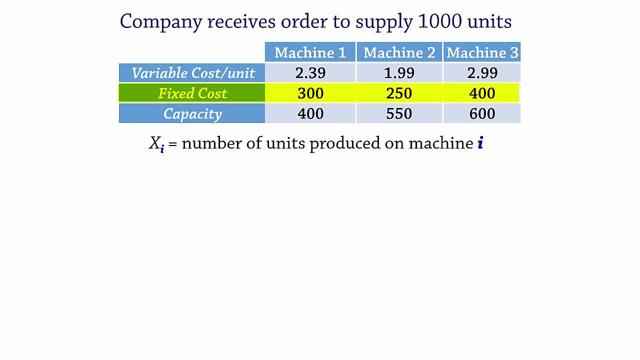 Now, because fixed costs indicate that the entire cost would be incurred if the corresponding machine is used to produce it all. we define another set of decision variables For machine 1. we can write: y1 equals 1 if machine 1 is used. 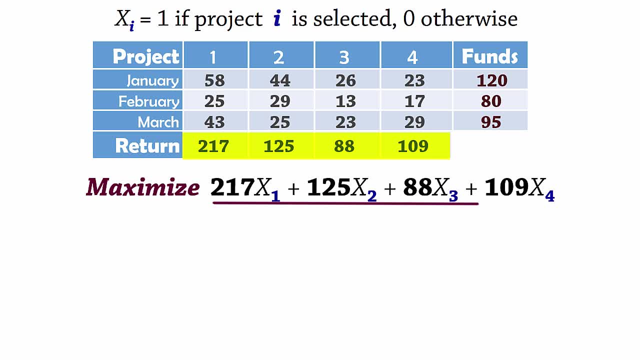 plus 125 X2 plus 88 X3 plus 109 X4.. Since project outlays are constrained by available funds, we write for January: 58 X1 plus 44 X2 plus 26 X3 plus 23 X4 less than or equal to 120.. 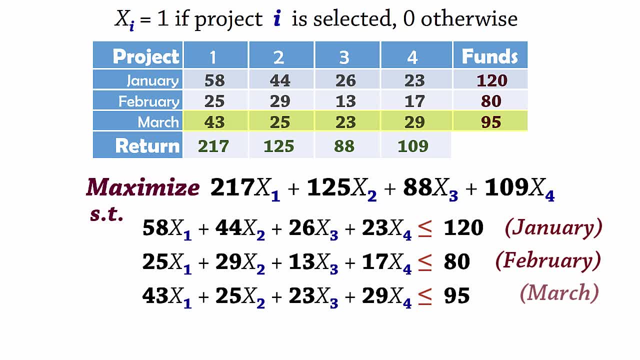 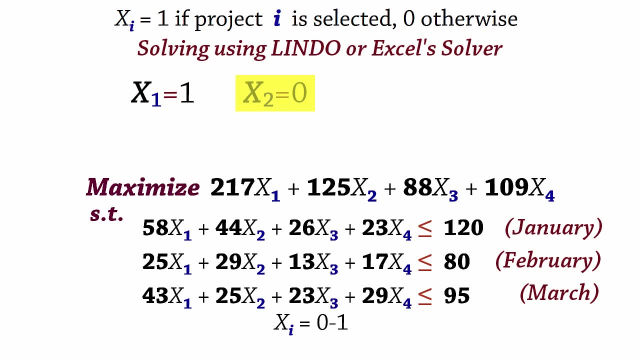 We do the same for February and for March, And then complete the model by stating that the decision variables must be binary. Upon solving this model using software like Lindo or Excel Solver, we find that the optimal solution is: X1 equals 1, X2 equals 0,. X3 equals 1,. 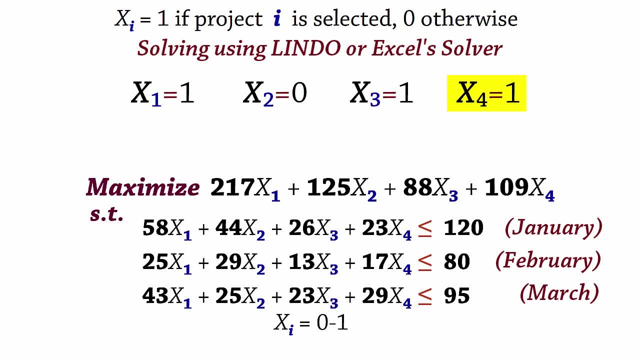 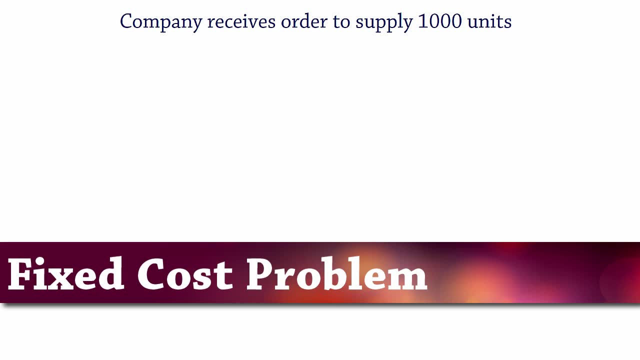 and X4 equals 1, with a corresponding net return of 414.. That is to maximize net return. undertake projects 1,, 3, and 4 only. Let's now model a fixed cost problem. Suppose a small company receives an order to supply 1000 units of a product. 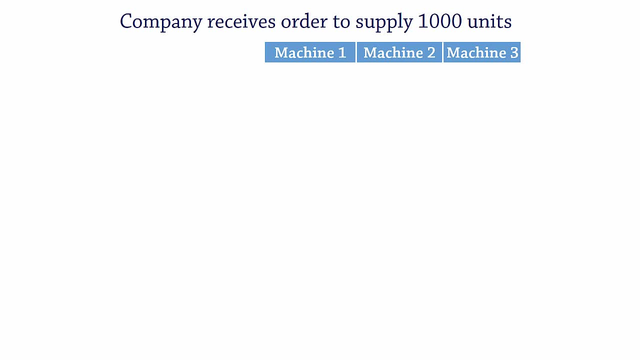 The company has three machines that can be used to produce the product. Here are the variable costs per unit produced from each machine, Here are the fixed costs and here are the machines capacities. Our objective is to minimize total costs. We are going to need two types of decision- variables in this case. 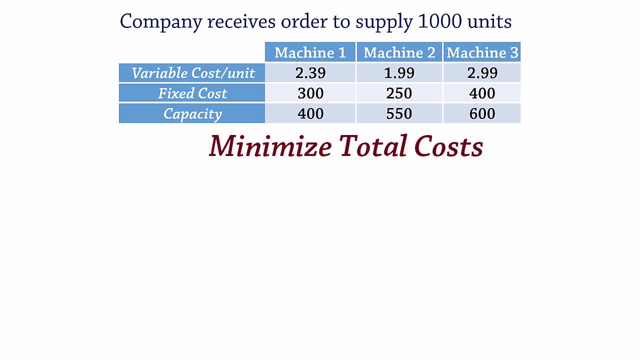 One set for the number of units produced from each machine and, because of the fixed costs, another to indicate whether a machine is being used or not. So for the units produced we write X. I equals number of units produced on machine I, That is, X1 represents the units produced on. 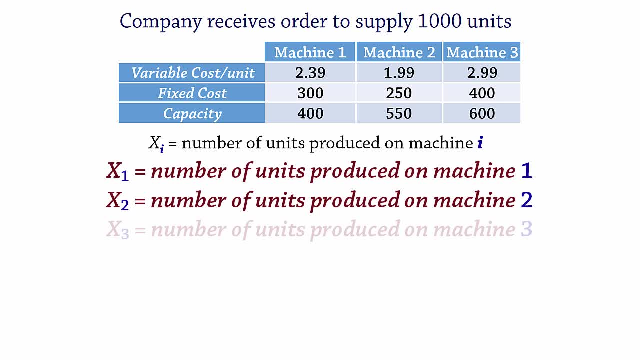 machine 1,, X2 for machine 2, and X3 for machine 3.. And here is the cost. We are going to need X2 for machine 3, X4 for machine 3, and X3 Mus for machine 9.. Now because fixed costs. 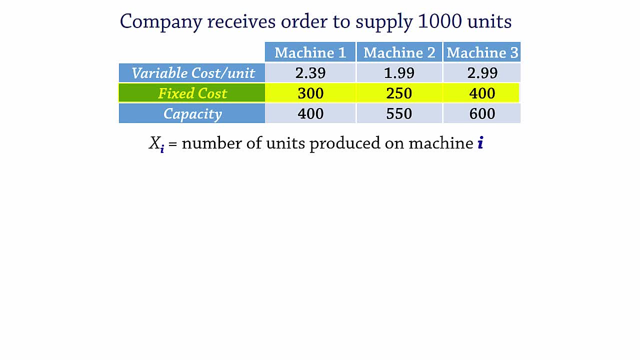 indicate that the entire cost will be incurred if the corresponding machine is used to produce it all. we define another set of decision variables For masvn1,. we can write: Y1 equals 1 if machine one is usedisierung, 0 if machine one is used otherwise. y1 equals 0 if X1 is greater than zero For all 3. 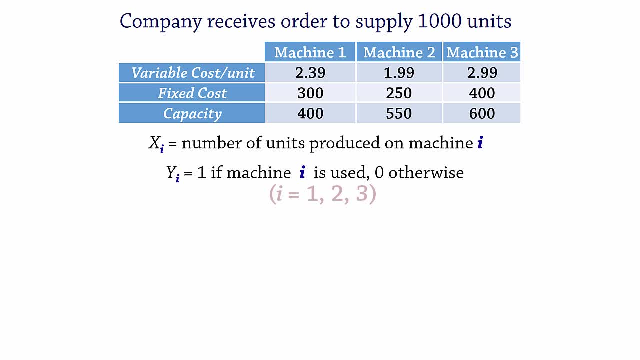 machines: we can write based on Y1 equal to 0 if machine one is used, ie X2 plus 1 if X2 is greater than 0.. machines: we write: y1 equals 1 if machine i is used, 0 otherwise. So for the objective function. 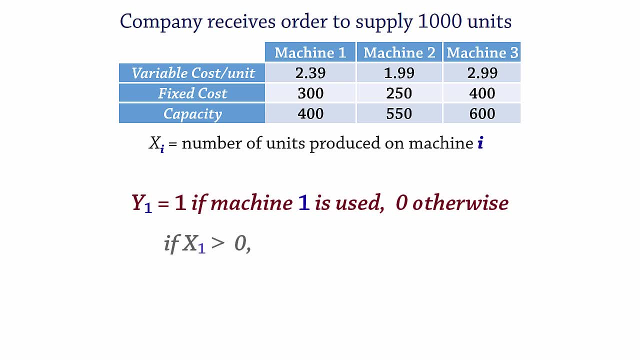 0 otherwise, That is, if x1 is greater than 0, y1 equals 1.. Otherwise y1 equals 0.. For all three machines we write: y1 equals 1 if machine i is used, 0 otherwise 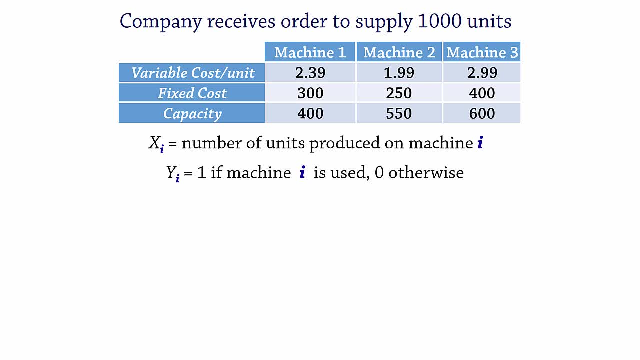 So for the objective function, which is to minimize total costs, we write: minimize 2.39x1 plus 1.99x2 plus 2.99x3 plus 300y1 plus 250y2 plus 400y3.. 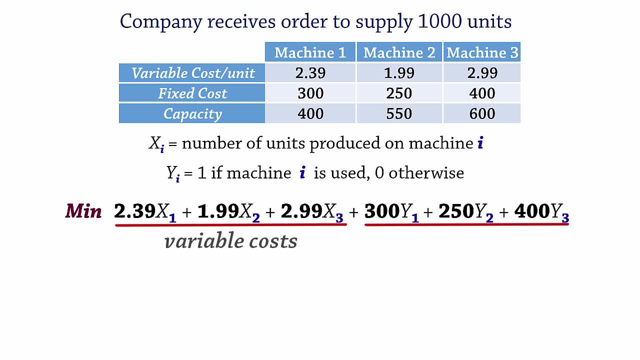 That is, we multiply variable costs by units produced and multiply fixed costs by the corresponding 0,1 variables. When y equals 1 here, for example, it means that machine 1 is used and the fixed cost of 300 will be incurred. 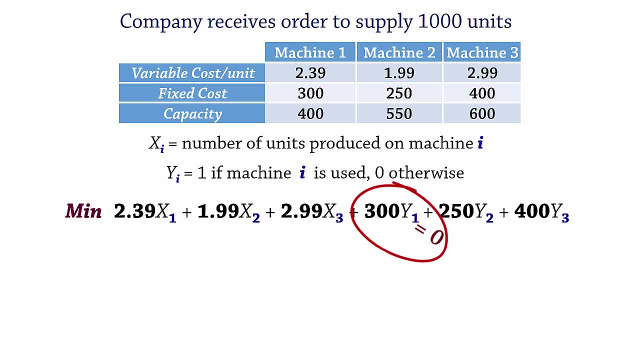 And when y1 equals 0, machine 1 is not used. so the fixed cost of 300 will not be incurred For the constraints. we have an order here to supply 1000 units. So we write: x1 plus x2 plus x3 equals 1.. 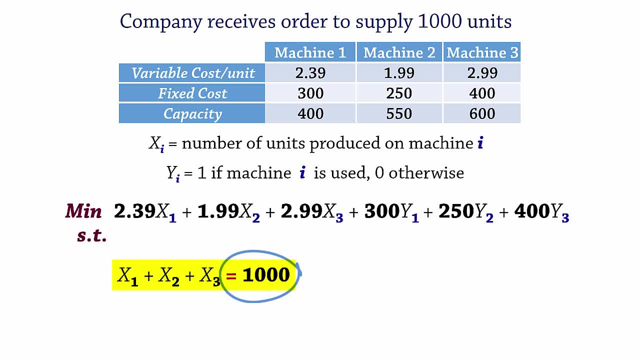 Equality is used here because we have to meet the order or demand placed by the customer. Now for the capacities. normally we just write x1 less than or equal to 400,, x2 less than or equal to 550, and x3 less than or equal to 600. 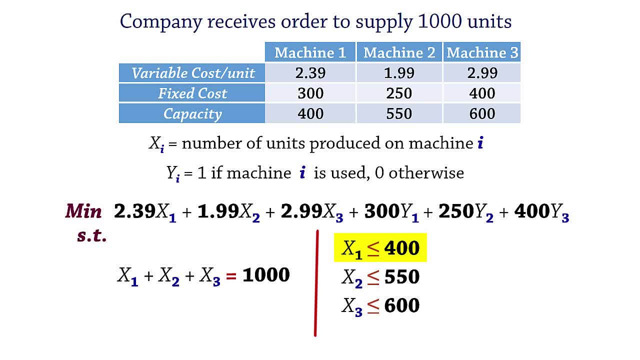 Note that this x1 less than or equal to 400 constraint simply states that we can produce up to 400 units on machine 1.. But if the machine is not used at all, this won't be possible. So whenever we have fixed costs associated with minimum requirements or maximum capacities, 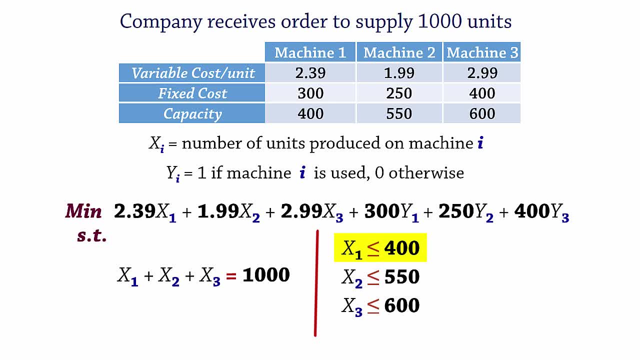 we usually multiply the capacity by the corresponding binary variable. So the correct format is x1 less than or equal to 400 y1.. That is, when y1 equals 1, we can produce up to 400 on machine 1, and when y1 equals. 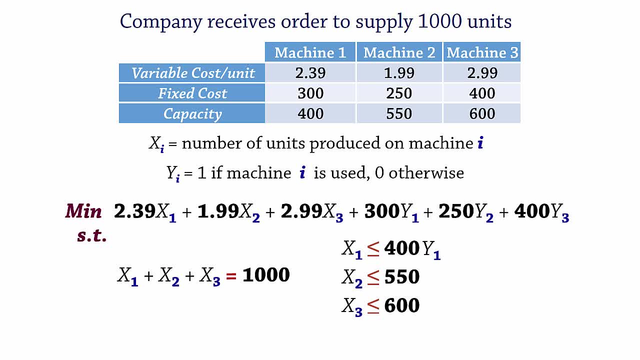 0,, 0 units should be produced. We do the same for machine 2 and machine 3.. We can then move the variables to the left side of the constraints and state that the xi should be non-negative and the yi is binary. 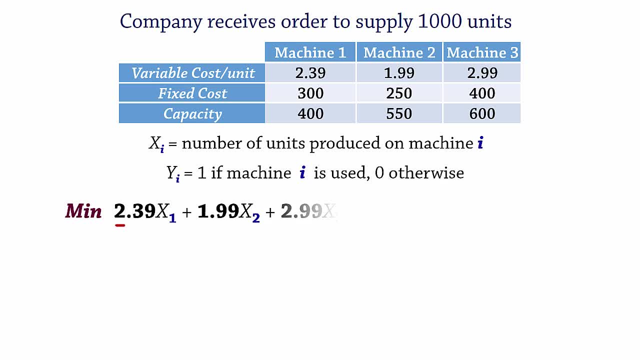 which is to minimize total costs. we write: minimize 2.39 x1 plus 1.99 x2 plus 2.99 x3 plus 300 y1 plus 250 y2 plus 400 y3.. That is, we multiply variable costs by unit produced and multiply. 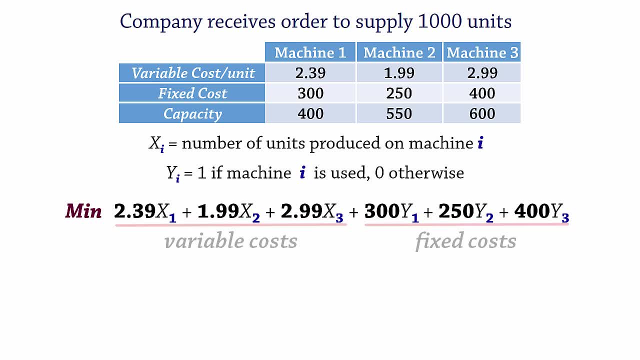 fixed cost by the corresponding 0- 1 variables. When y equals 1, here for example, it means that machine 1 is used and the fixed cost of 300 will be incurred. and when y1 equals 0, machine 1 is not used, so the fixed cost of 300 will not be incurred. For the constraints, we have an order. 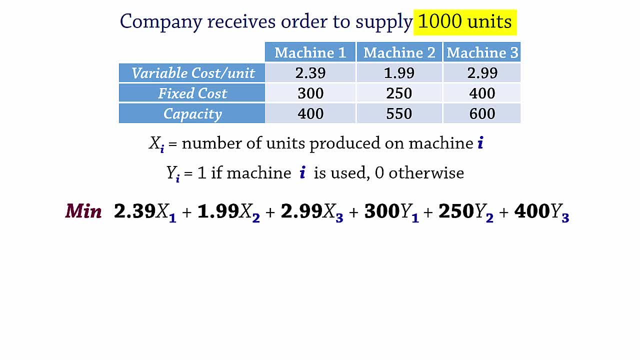 here to supply 1000 units. so we write: x1 plus x2 plus x3 equals 1000.. Equality is used here because we have to meet the limitations of our machine. 1. the x1 is used here to supply 1000 units, so we: 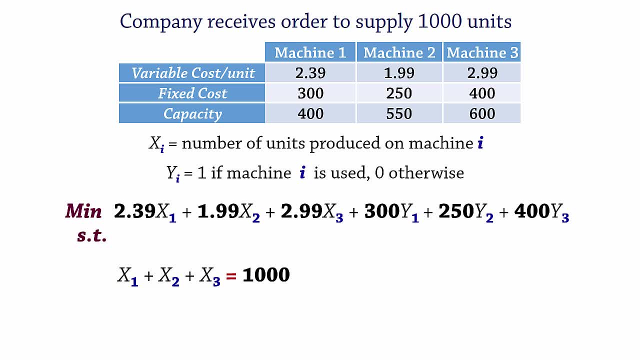 the order or demand placed by the customer. Now for the capacities. normally we just write X1 less than or equal to 400, X2 less than or equal to 550, and X3 less than or equal to 600.. Note that this X1 less than or equal to 400 constraint simply states that we can produce. 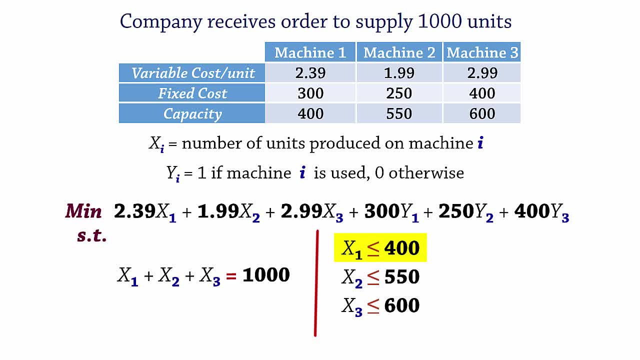 up to 400 units on machine 1.. But if the machine is not used at all, this won't be possible. So whenever we have fees, costs associated with minimum requirements or maximum capacities, we usually multiply the capacity by the corresponding binary variable. 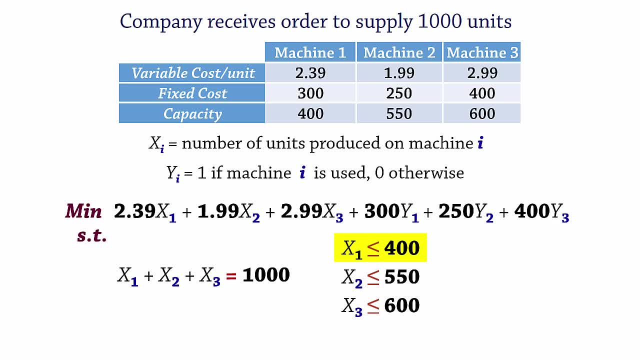 So the correct format is X1 less than or equal to 400 Y1. That is, when Y1 equals 1,, we can produce up to 400 on machine 1, and when Y1 equals 0,, 0 units should be produced. 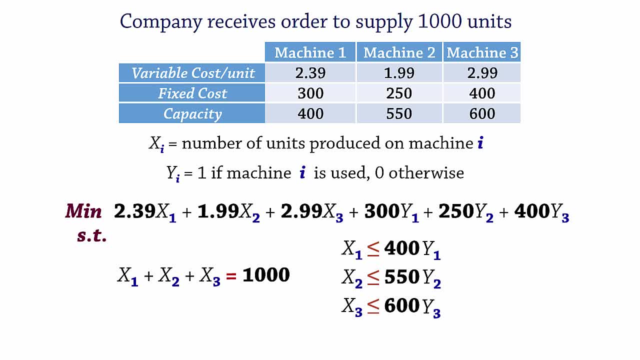 We do the same for machine 2 and machine 3.. We can then move them to machine 3.. We move the variables to the left side of the constraints and state that the XI should be non-negative and the YI is binary. 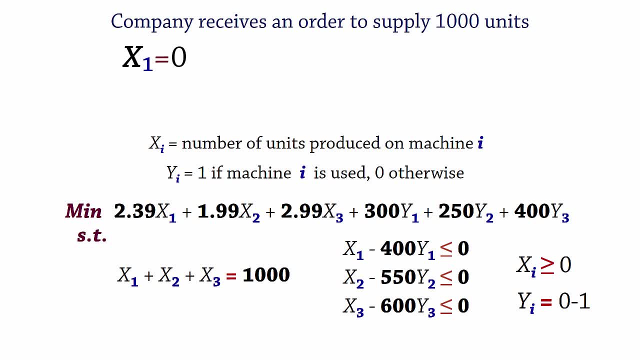 On solving this model, we obtain: X1 equals 0,, X2 equals 550,, X3 equals 450. And for the binary variables, Y1 equals 0,, Y2 equals 1, and Y3 equals 1, showing that: 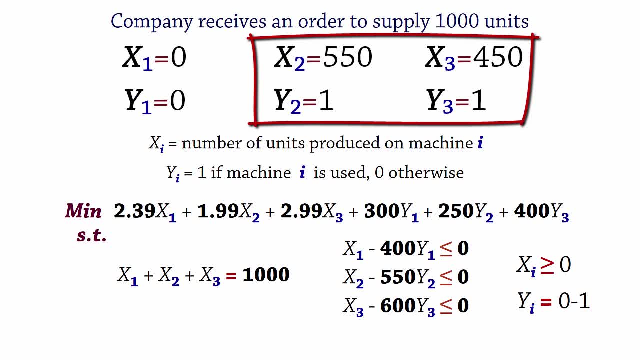 only machines 2 and 3 should be used. And that completes this fees cost problem. In the next video I will be showing you how to solve the fees cost problem. I will be showing how to formulate some relational constraints using binary variables, including.